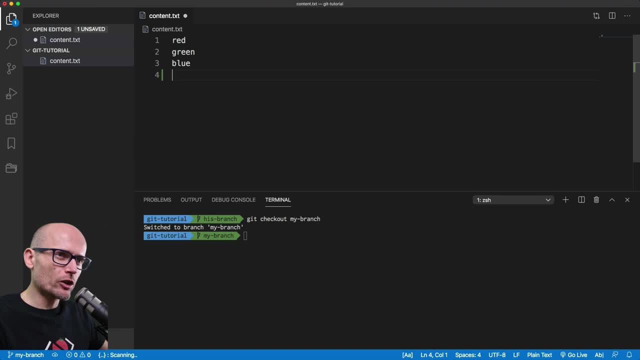 and we'll save it as his changes and in my branch I will add two colors and save it as commit with the message of my colors or my changes. Now we can try to merge his branch into my branch. Let's say, I'm working on a feature and your colleague is working on another feature and 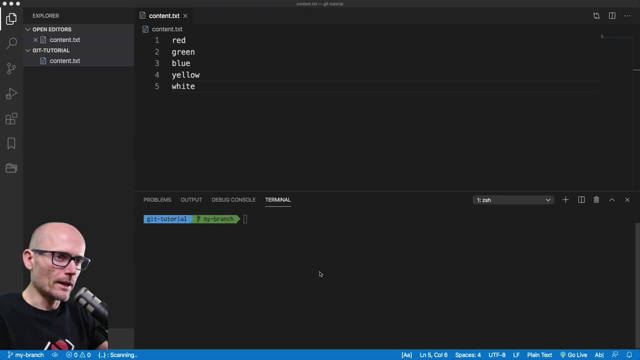 you want to bring his feature into yours and continue working in your branch? Okay, so we will try to merge his branch into my branch, And to do that we simply need to check out the branch you want to merge into. So we are currently. 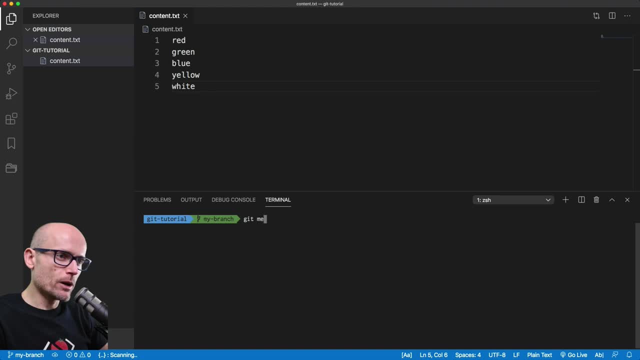 on my branch, which is correct, and we want to merge his branch, Okay. so remember, you need to be checked out on the branch you want to merge into and then you merge the branch of the changes you want to bring in, Okay, so if we do that, then you will definitely get a conflict, because we both 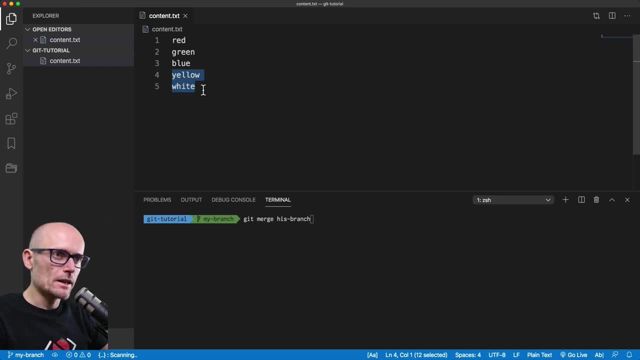 edit the lines four and five of the contenttxt and then Git doesn't know how to automatically resolve this conflict because we both touch the same file in the same lines. If we touch different lines then Git could easily merge it automatically, But because we've edited the 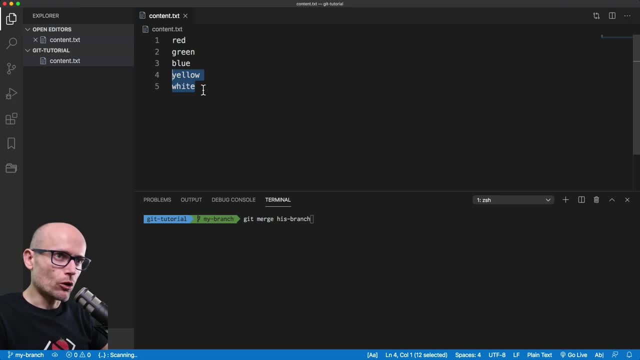 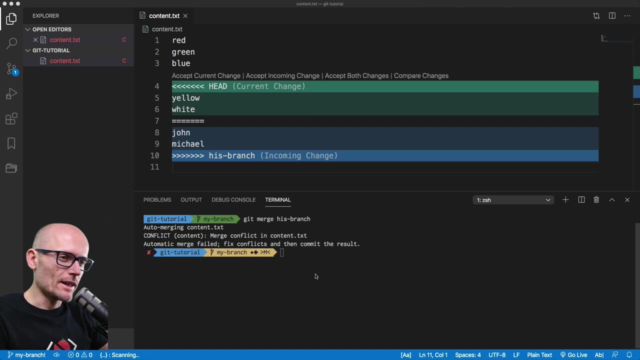 same file, same line, we gonna get conflict, And here it is the famous conflict that everyone hates and we, in this tutorial we are going to create, you will learn how to resolve it without any headaches. so we are being notified by git that the content txt is the issue and he couldn't automatically resolve it, and we need to resolve. 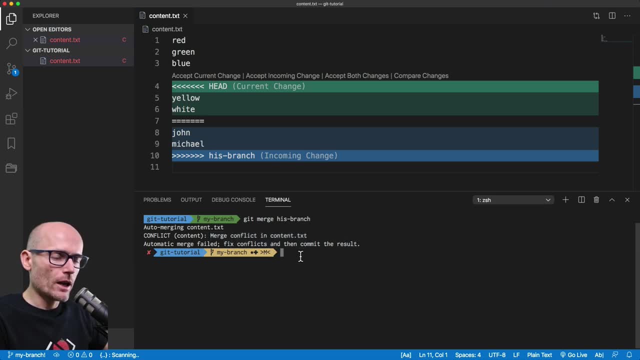 the conflict manually and commit the result. okay. so if you freak out at this moment and decide to quit the merge, call ambulance or policemen or firefighters, whatever your approach is- then you can still revert back to merge. so abort the merge and the command is: git, merge, abort. 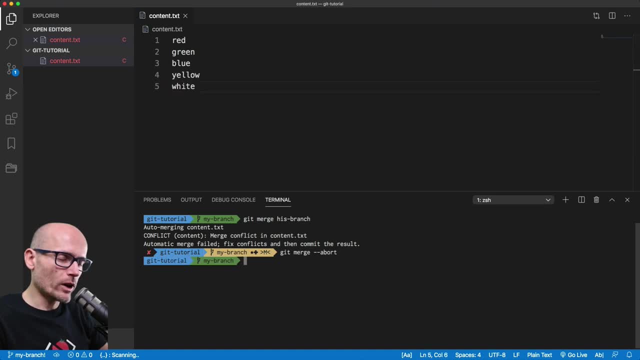 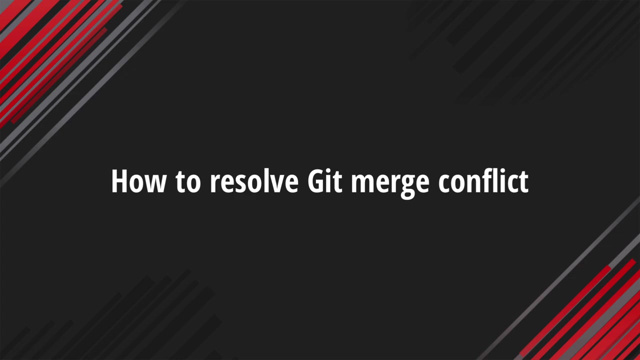 okay, that will revert the merge, cancel everything and you are back where you were before merging these two branches together. so if you freak out, the abort will always get you out of trouble. now we try to be brave and we will merge so we can go back to the. 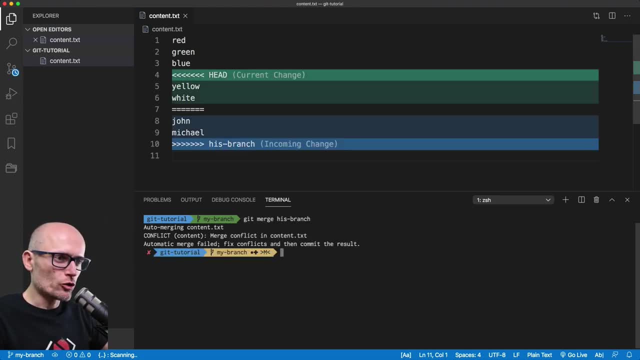 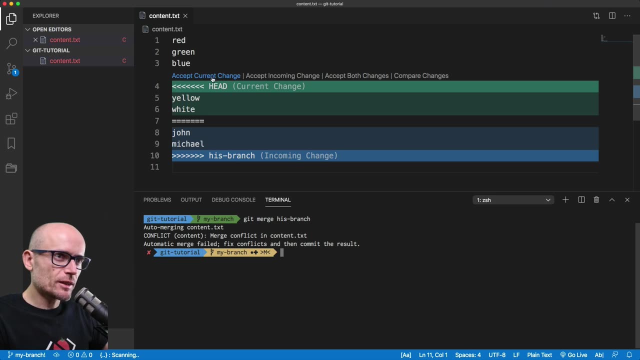 and merge again, and this time we'll try to resolve it. we won't be aborting, we will be resolving, okay? so we've got a couple options here. the first one is accept the current change, which is the change in your branch, or in this case my branch. then the accept incoming change, which would only take the 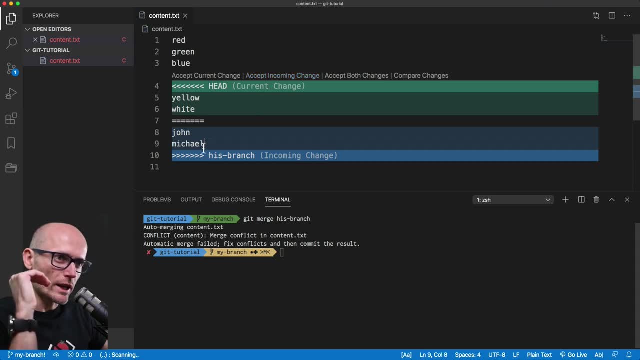 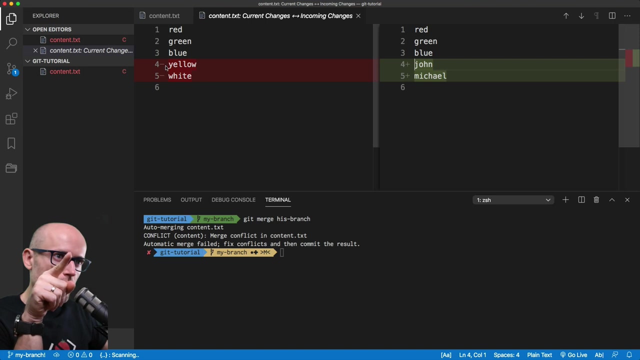 changes the incoming changes, which is the john and michael, or we can accept both, which would keep the file and write all these four lines into it, or we can compare the changes. so here is the change visually: on the left we are adding yellow, white. on the right side we are adding john and michael. so this is the two files side by side. 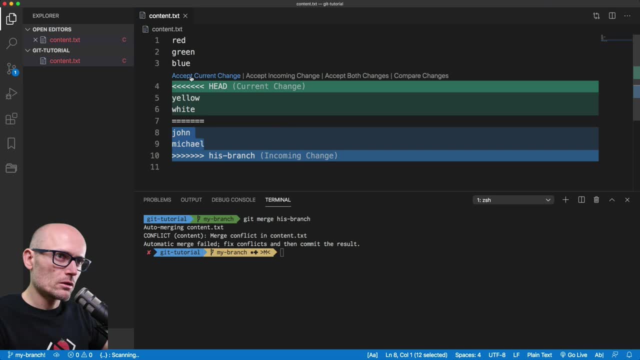 and it's up to us how we want to resolve it. i will first accept the current change, which would bring the two colors. if i revert it, accept incoming change, john and michael comes in again undo it, and if we accept both, we see all four lines written. okay. so this is the three options you have and it's up to you how you resolve. 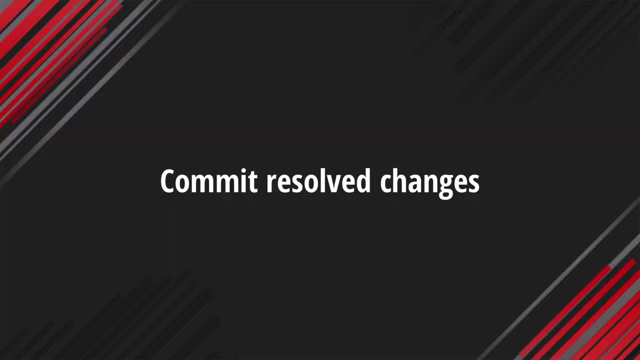 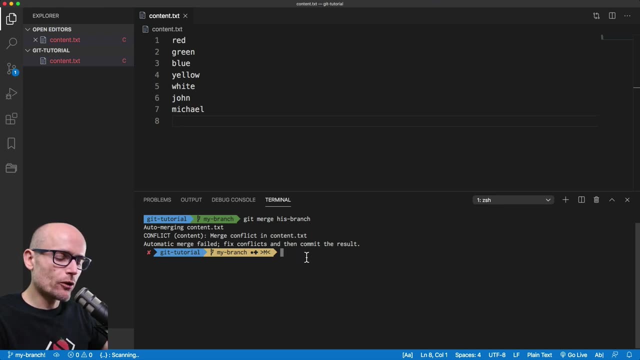 it based on your code. we will save the file with the changes we are happy with and at that moment, we are still in the merge process. okay, so if we look at git status, you see that we have unmerged pass, which means that this file is still not resolved. we need to mark it as. 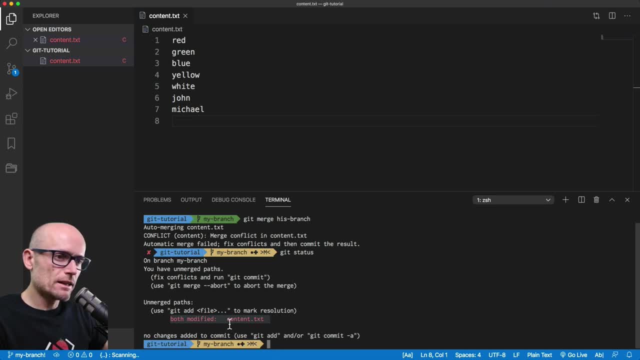 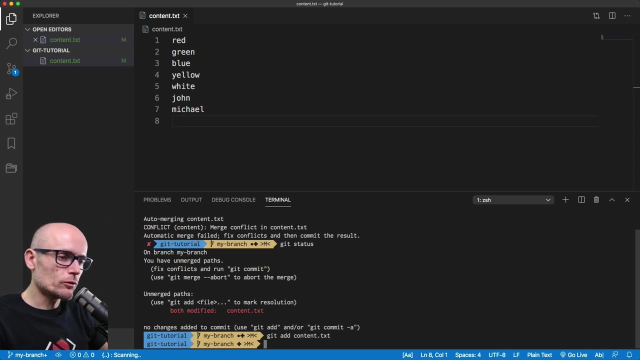 resolved and to do that we need to use the git add and the file name. okay, so if we go git add and contenttxt or git add dot or period, it will do the same thing. that tells git that that file is resolved and now we can commit it. and we can simply git commit and give it a clear message. 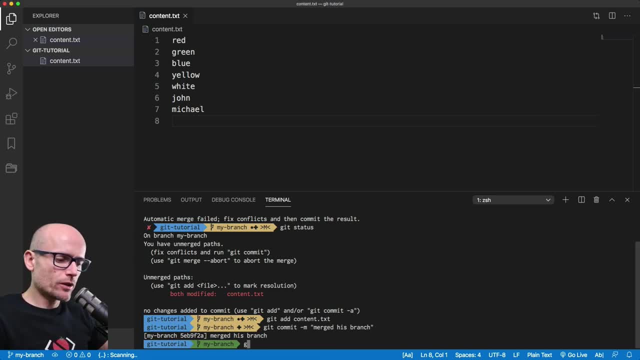 merge to his branch. now the changes are merged, git status should be happy and git log should show us that we have the merged his branch commit successfully completed. and that's how you resolve conflicts in git. I know it can be frustrating when you're merging and having conflicts, but only practice makes you perfect, so don't be afraid to create a simple demo.